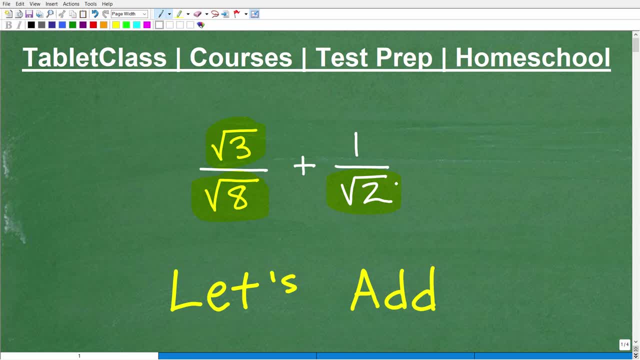 Okay. so we're going to talk about that. We're going to talk about how to do this problem, And I'm actually going to do it in two ways, Okay, two ways that you're certainly going to want to know how to do. Of course, ultimately, you know you need to get the right answer. If you want to turn this into a little pop quiz- pop, you know, by pause in a video and see if you can get the right answer, that would be excellent. But I'm going to get into exactly what we need to do here, step by step, in just one second. But first let me quickly introduce myself. My name is John. I'm the founder of Tablet Class Math. I'm also a middle and high school math teacher. 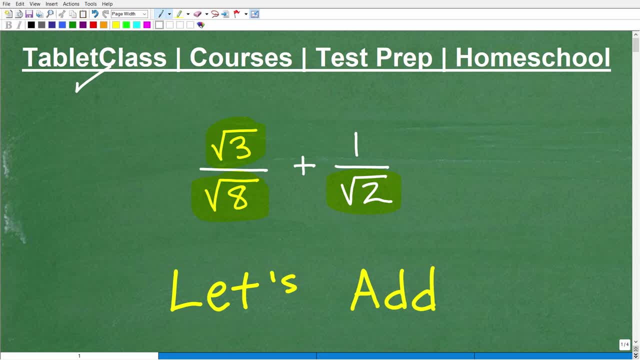 And I have an excellent math help program. Let me just tell you very briefly what it contains Basically. I have 100 plus different math courses ranging from pre-algebra to pre-calculus and everything in between. I also have a ton of test prep courses. So if you're taking an exam and it has math on it, I likely have a test prep course for it. So I'm talking about, like the GED, SAT, ACT, CLEP exam, ACCUPLACE or ALEC exam, a teacher certification exam, ASVAB, GRE. you kind of get the idea. 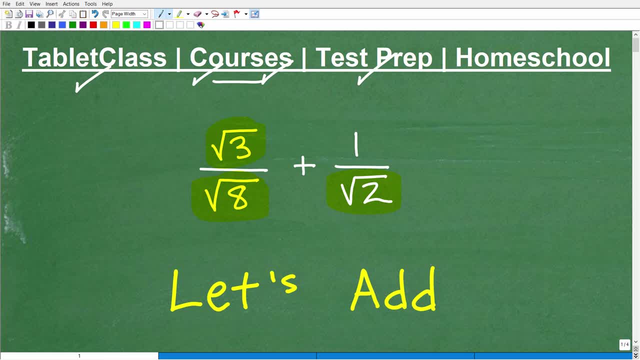 Right. So there's a lot of exams people have to take And quite often there is a math section on these exams. So just go to my my site. Of course, I'm going to leave the link to my site and the course in the description of this video, But I also do a lot with homeschooling as well. So if you homeschool, I have a great homeschool math learning program And then obviously help those of you who are having a tough time in your current math courses. So that's a little bit about my program. One thing I must say is this: If you are a math student and your notes are anything less than outstanding, 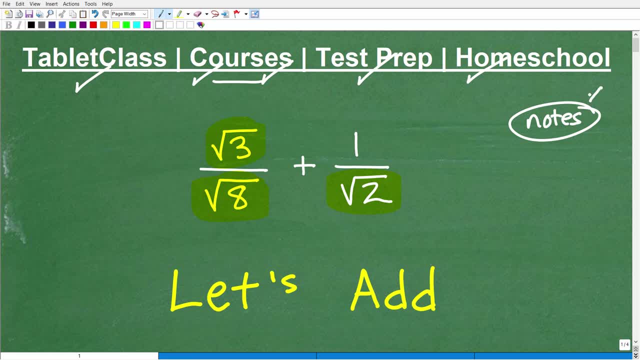 you need to work on your notes. I've been teaching math for decades. This is critical. OK, so take great math notes and great things will happen. But in the meantime, you can use my notes to study from. I'm going to leave links to those and links to all this stuff in the description of this video. 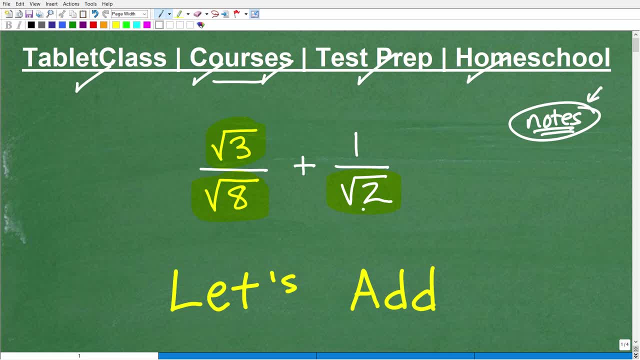 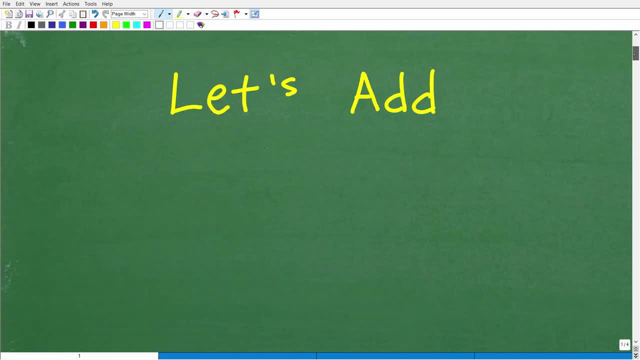 OK. so if you think you can add these up and get the final correct answer, go ahead and try. OK, I certainly encourage you to do so, or at least think about it. But let's just talk about fractions in general. Now this problem: one half plus two thirds- OK, so here's a fraction problem. Now, what comes to mind? OK, for the most people, you're thinking: I need to get that LCD. OK, the lowest common denominator, Because, remember, these denominators must be the same in order for us to add these fractions. So that's good thinking And that is correct. Now, what is LCD for this particular problem? Now, if you said: 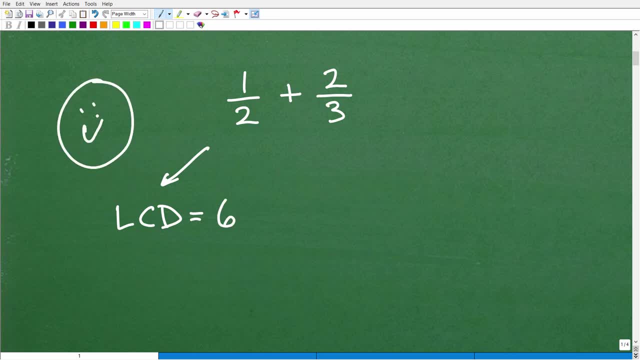 six, then I must reward you with a nice little happy face. OK, so nice job. That is correct. The LCD is six. So I'm going to have to rewrite each of these fractions, OK, such that the lowest common denominator six, then add them up and reduce and simplify. OK. so that is very important, Matter of fact. let's just do that very, very briefly, briefly. So let's change this. Let's see, we have to multiply this by three, the denominator by three and the numerator by three. 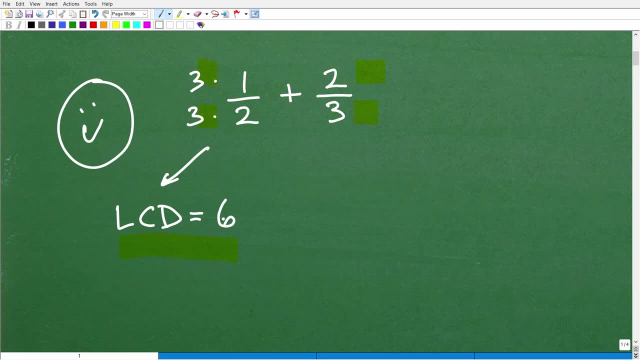 To get six. Now the reason why the LCD is six, that's a whole separate discussion. I have done a ton of videos on how to find the LCD and fractions, So if you're struggling with fractions, you know just basic fractions. just check out my pre-algebra playlist. Some of my videos on my fraction videos and LCD videos literally have like a million plus views. So there's a lot of people looking for fraction helps. So don't be shy about reviewing fractions. A lot of people need to. OK, so here I have to multiply this by three. 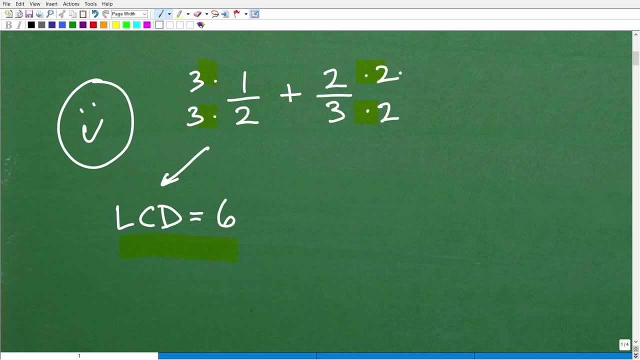 I have to multiply this by two. to get a six, I have to multiply this by two. I'm skipping over a lot of stuff, but I think most people, hopefully, will get the idea. All right. So this fraction here now will become three over six. plus this fraction will be four over six. Now I can add the numerators. OK, so this would be seven over six, because now I have the same denominator. OK, so that's basically what we're going to be doing And this is the same steps that we need to apply. 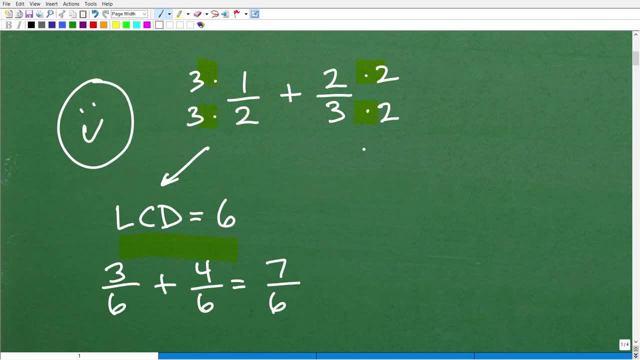 For this particular problem. OK, so you need to know how to do this. Now there is a another way. OK, I call this one of the best fraction hacks out there, And it's called for. the way I call it is a bow tie method. OK, this is something you absolutely need to know. OK, so let's go ahead and see how this works. All right, So we know? the answer is seven over six. So let's talk about the bow tie method And I'll draw a little bow tie here. It's a little hack. This will be a different way We'll do this problem. 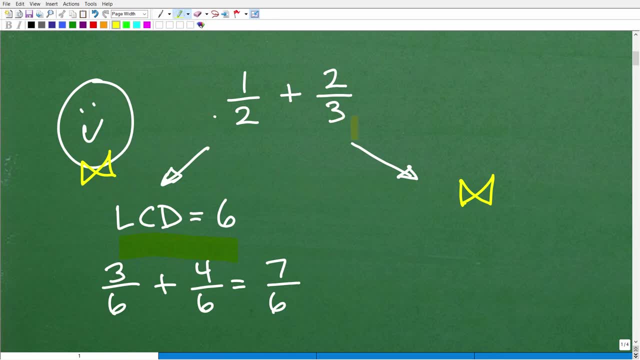 So this is how this works. OK, Now again, this is just a quick, quick review. You want to you know more thoroughly? practice this. OK, my other videos. But here, here's how it works. You start from the bottom right and you multiply up, OK, so, so the bottom right, that's the denominator. And it's not this way, It's this way, It's exactly this way. So three times one is three. Now this is an addition problem, So that's going to be plus. OK, what I'm forming here is my numerator. 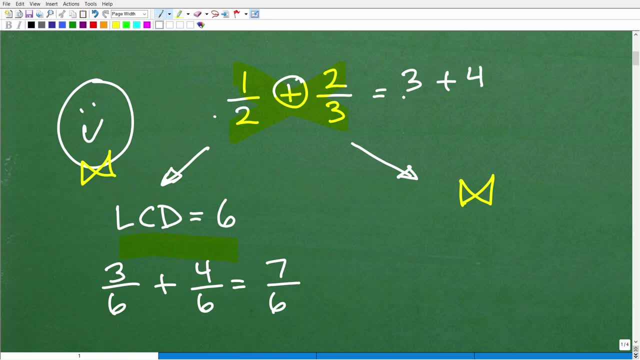 Two times two is four. OK, now that right there, just forms my numerator, And to get my denominator, it's going to be two times three. Just multiply this times this, That's six, And look at there, We have seven over six. Look how easy that was. OK, so you have two methods to add fractions, And this particular method is awesome. However, sometimes you don't end up with the lowest common denominator, So you might end up reducing at the end. 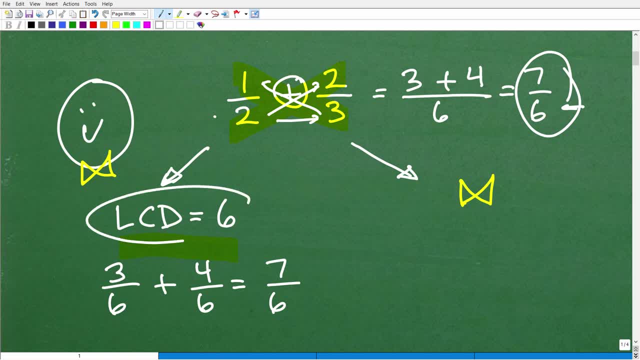 OK, but you definitely will get the problem right. OK, so again, we can get our LCD, or we can just jump right into the bow tie method. You really should know how to do both when it comes to fractions. OK, All right. So now let's get into our problem. 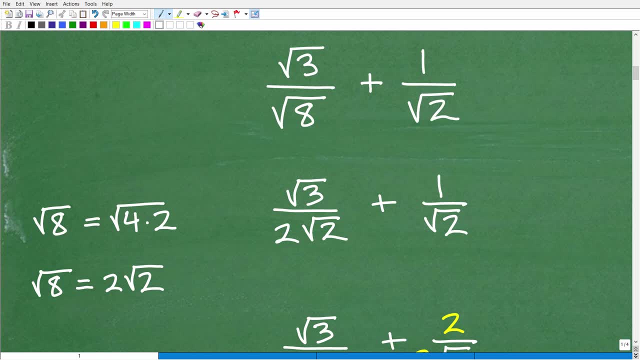 OK, so here I have the square root of eight and a square root of two. Of course I'm going to add these up, But there are clearly, you know, these denominators are not the same. Now I can't really determine the value of this or can't compare these. 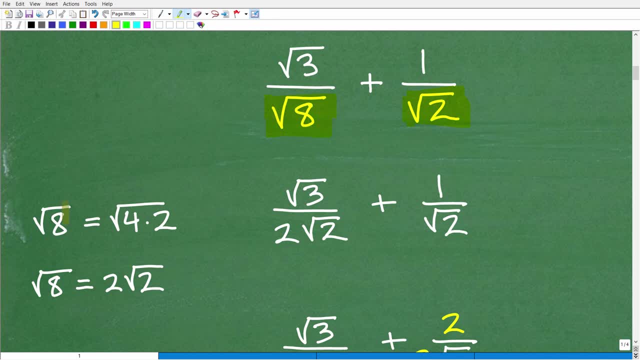 Yet, because the square root of eight I can simplify OK, so you should know how to do this. If you don't know how to do this, you want to look at how to simplify square roots or simplify radicals. It's very, very important. So the square root of eight is equal to the square root of four times two, because four times two is eight. 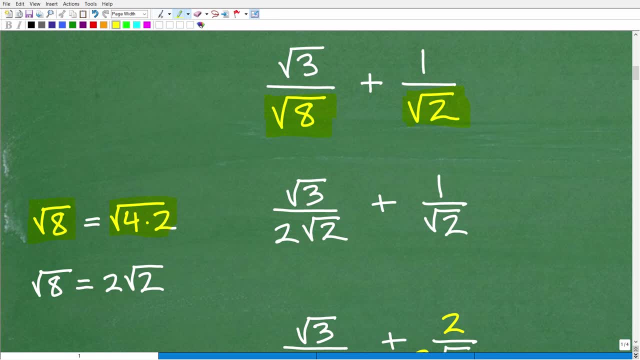 So the square root of eight is the same thing as a square root of four times two. Now, one thing you could do when you have square roots is split them up. So this is the same thing as the square root of four times the square root of two. 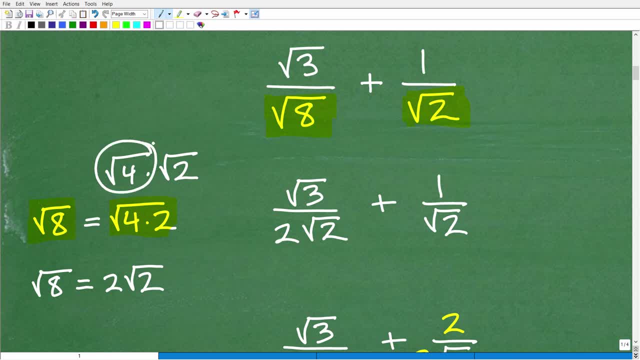 And that works out nicely for us, because we know that the square root of four is two. OK, so that's two, And it could be positive or negative two, But for right now we'll just keep it simple. So it's going to be two times the square root of two. OK, so the square root of eight is equal to two times the square root of two. 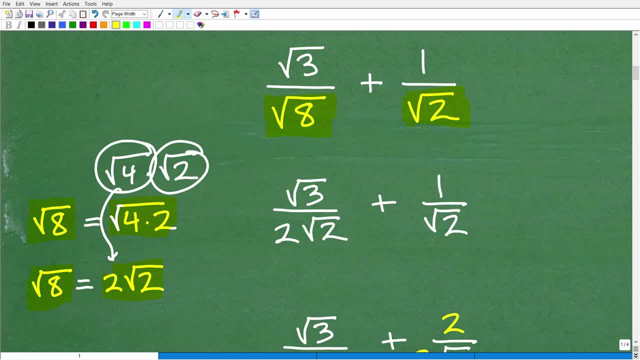 We need to know, understand that, because once I have the square root of eight written, and it's simple as four, OK, which is two times the square root of two. So here's my problem: OK, the square root of eight is two times the square root of two, I can more easily identify the LCD. 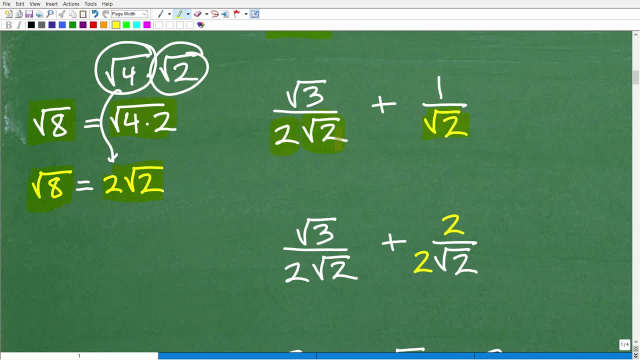 OK, so what is the LCD? Well, if I have a square root of two, and this is two times the square root of two, it would be pretty easy if I just multiply this by two, because that would be two times the square root of two. 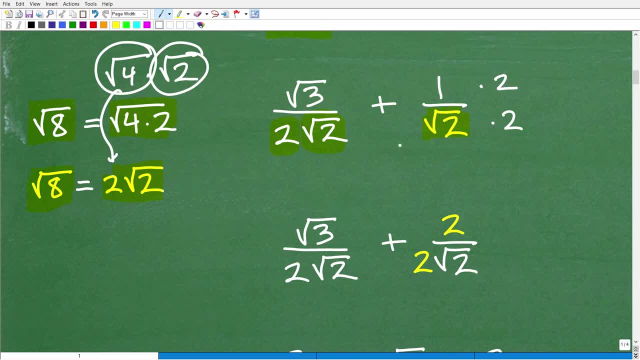 And then I could just multiply the numerator by two. So in other words, two square root of two is LCD. So I'm going to multiply this by two, OK, so I can have a Two square root of two. So if I do that, I'm going to have to multiply the numerator by two. 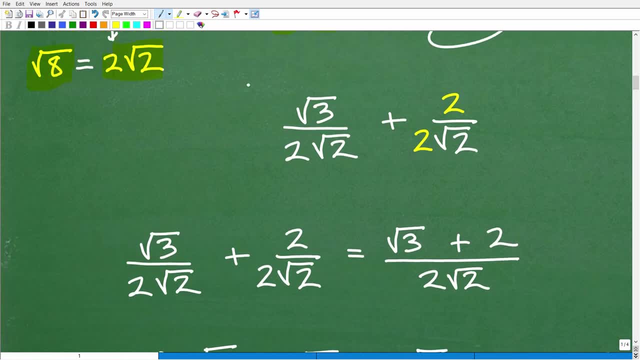 OK, so you can see that step right here. So now the problem is: square root of three over two, square root of two. Remember, we simplified square root of eight plus two over two square root of two. Now my denominators are the same. I have my lowest common denominators. 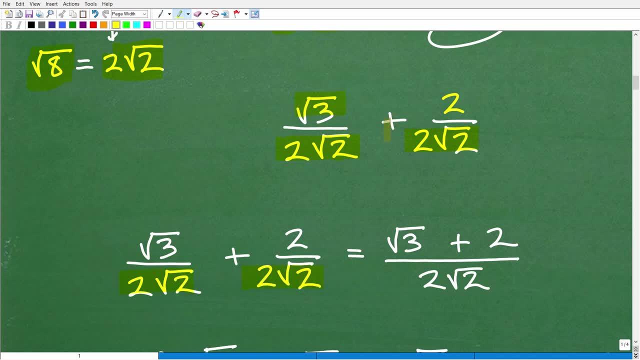 So now I can simply just add the numerator. So that's going to be the square root of three. I'll do it over here: Square root of three plus two. Square root of three plus two over two. square root of two. That is the answer. OK. however, matter of fact, how many of you got that right? 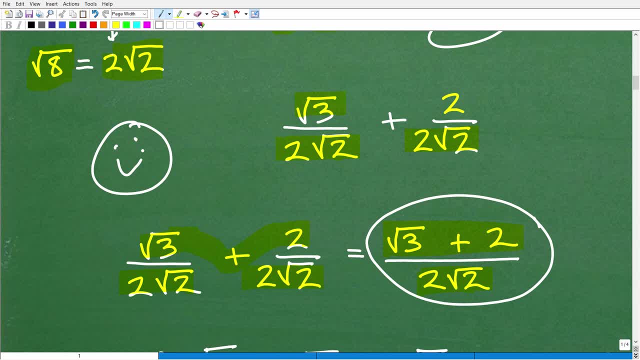 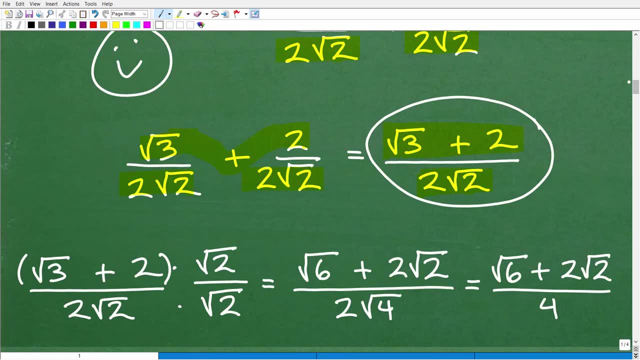 If you got that, I will in fact give you a happy face. I'm not going to give you an A plus or 100 percent, because we are not done. OK now, why are? why is this an issue? Well, in the denominator we have a square root. 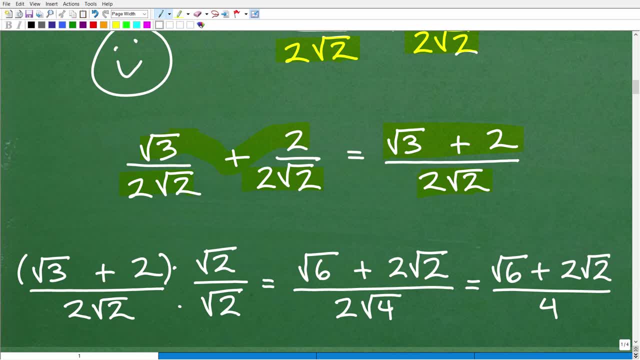 We have what we call an irrational number, The square root of two. we're not allowed to leave that down there. We have to do something called Rationalize. OK, now, that's a whole nother topic. OK, so you can see, this problem is: you know quite, you know there's other like skills you need to know, especially with square roots. 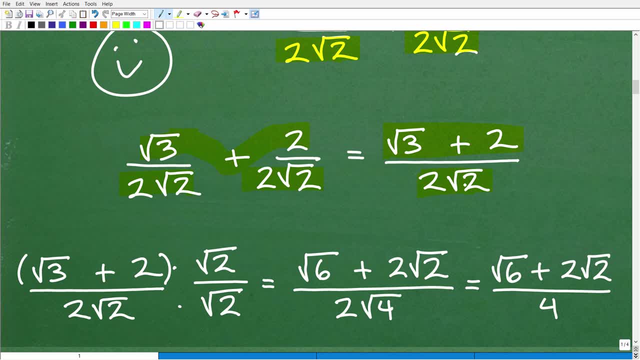 You're going to need to know how to simplify square roots and rationalize square roots and find the conjugate. So all this stuff you can continue to learn by checking out my pre-algebra, algebra and playlists, or just maybe just sign up for my algebra one course. 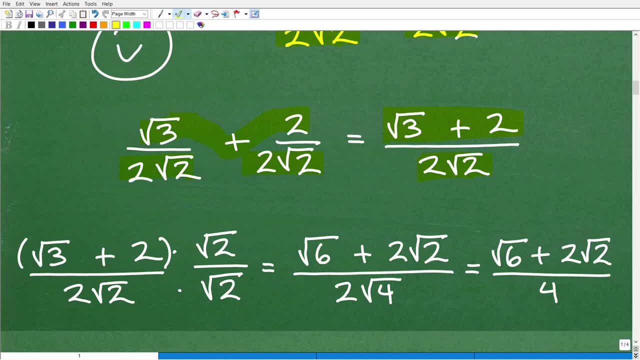 Whatever level of algebra you might be in, I certainly could teach you this in a very, very thorough manner. OK, so here's what we need to do. Again, I'm not going to fully explain this, but if I want to get rid of this square root of two down here, I can multiply. 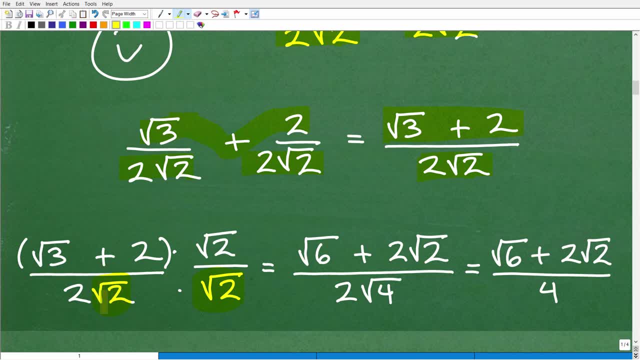 What you do is just multiply by this radical. So if it's a square root of two, I'm going to multiply it by a square root of two. That'll get rid of it. But if I multiply the denominator by a square root of two, I have to multiply the numerator by a square root of two. 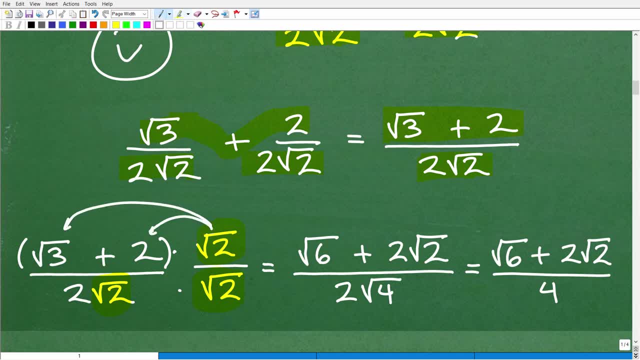 Now I have to use a distributive property to multiply. So the square root of two times square root of three, right there is a square root of six. square root of two times Two is two square root of two. Now I have my denominator two times. square root of two times square root of two is square root of four. 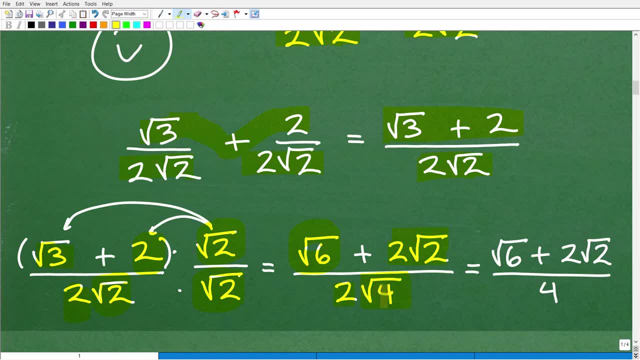 So I have two square root of four. Now I can get rid of that square root of four. That's just going to be two. OK, this becomes two. square root of four is two. Of course it's positive and negative. We'll just keep it nice and easy. 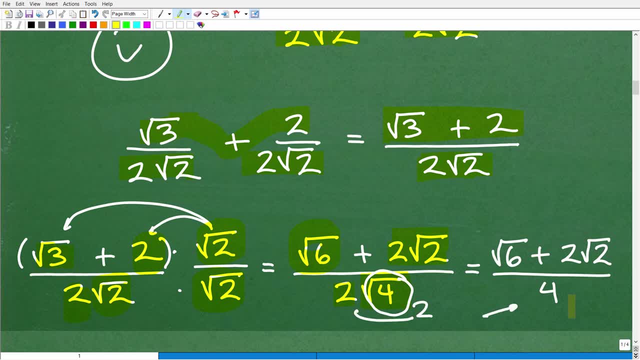 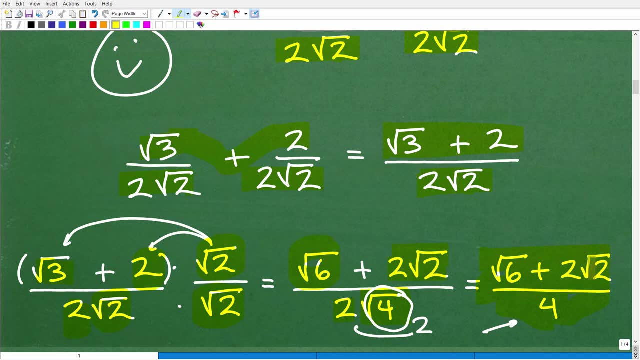 So that's two times two, which is in fact four. OK, and here now is your final answer. Now, if you got this right square root of six plus two Over times the square root of two over four, then I definitely will give you an A plus a one hundred percent. 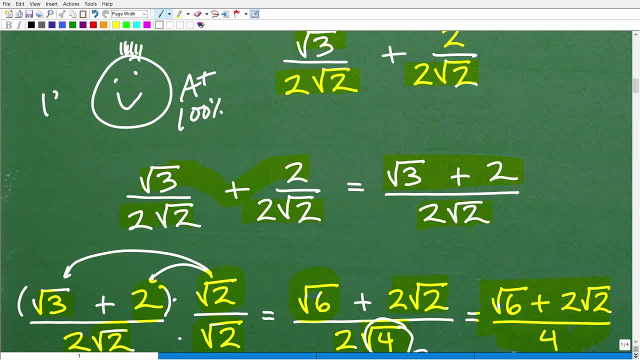 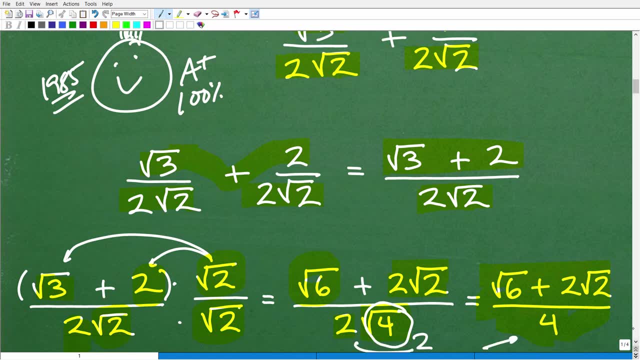 And, matter of fact, I might give you a nineteen, eighty, five flat top haircut. OK, that was a pretty cool haircut. I don't know why nobody wears those anymore, but I thought that haircut was pretty cool. Anyways, let's move on with the prom. 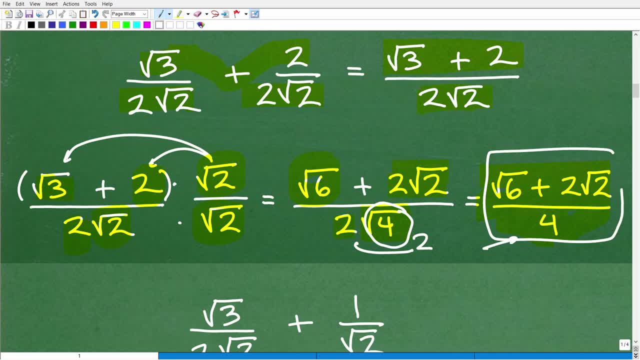 So you can see, this is a fair amount of work. All right To get our answer. All right, What do we have to do? We had to, you know, simplify The square root of eight. We had to find the LCD. 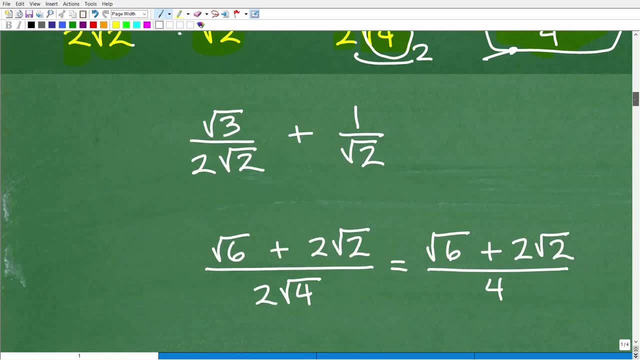 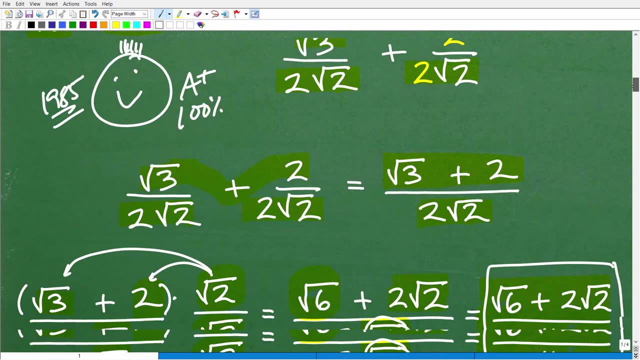 We had end up rationalizing. But now let's use our knowledge of the bow tie method. This first method here was using the LCD. OK, we found the lowest common denominator and we got the answer. All right, Now let's use that bow tie method and see if this is a little bit easier. 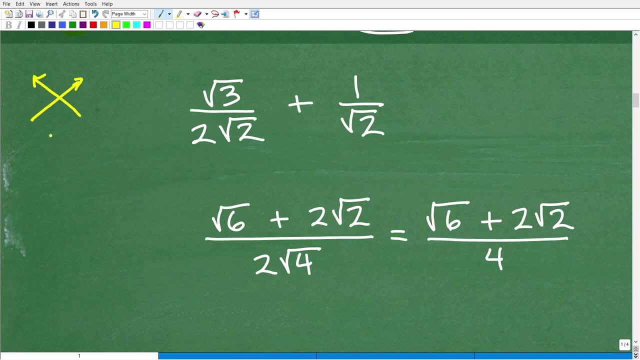 OK, remember it's this times, this times, this times, this over, this times, this. OK, so you can see how it goes here We're going to start from the bottom right. Square root of two, Square root of two times a square root of three. 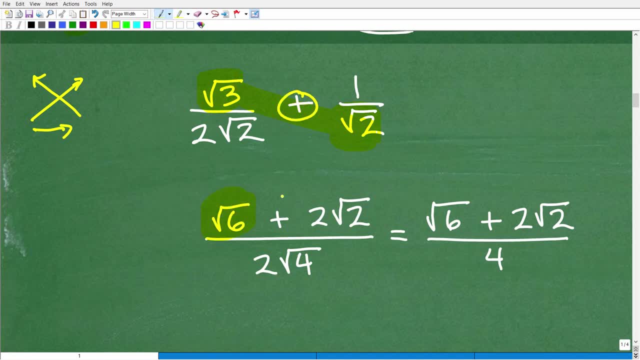 That's the square root six. This is an addition problem. OK, so that's going to be a plus sign right there. Then I'm going to have two tensors: square root of two times one, Well, two times two times the square root two. 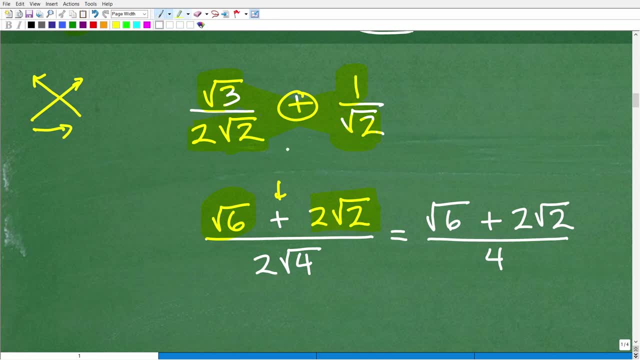 Times one is nothing but two times a square root, two. And then my denominator is going to be two times the square root, two times the square degree to two. So this is going to be square two times quarter two. That is going to be the square root of four. 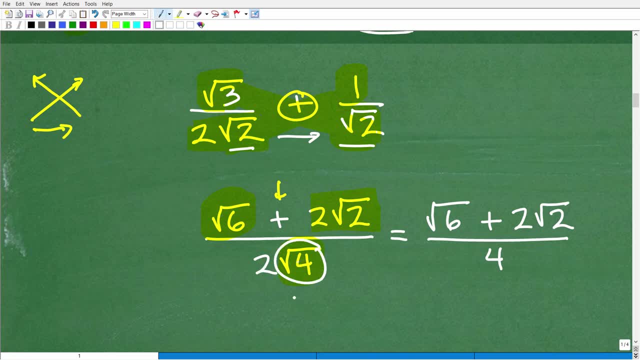 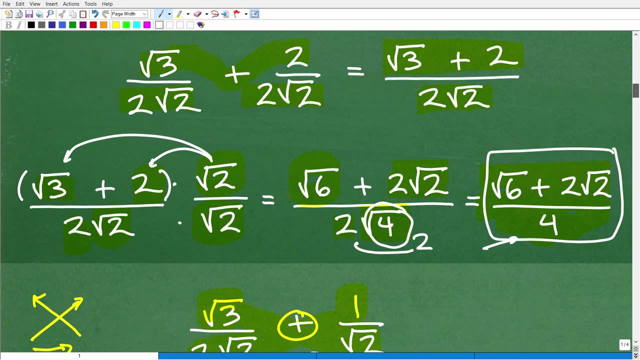 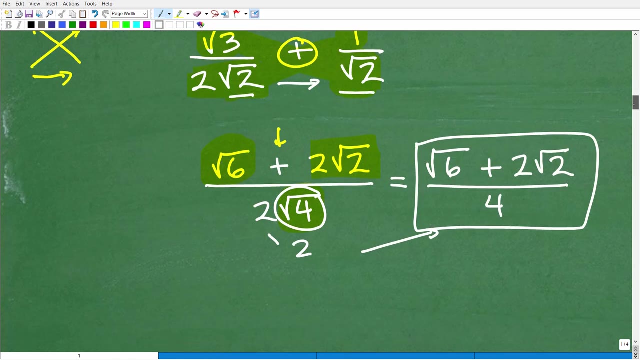 So I have to square root of four. Again, 4 is 2.. 2 times 2 is 4.. I am done. Okay, Now look at our answers. Square root of 6 plus 2, square root of 2.. Square root of 6 plus 2, square root of 2 over 4.. Okay, And this one's over 4.. They are: 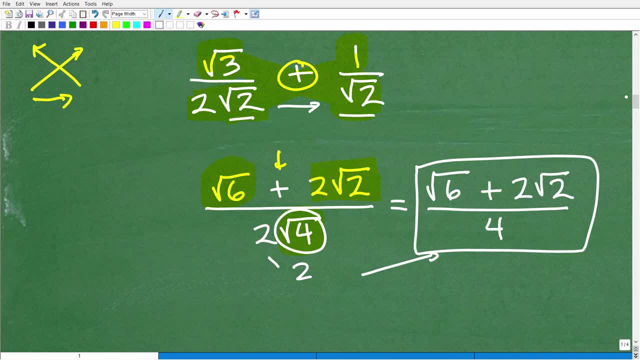 the same answer: Okay, So this method is awesome. Now you need to know both. You need to know how to work with the LCD and you need to know how to simplify radicals and rationalize radicals as well. These are critical skills, But you know, this is also an opportunity for you to see the 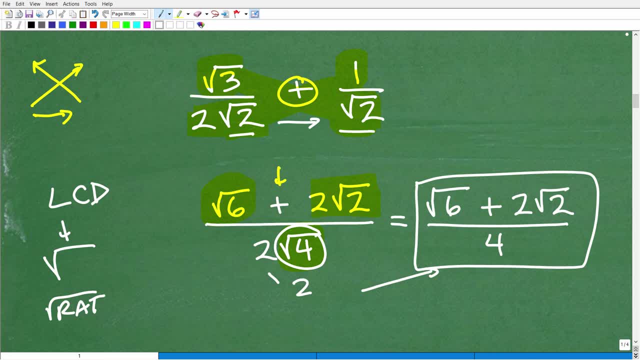 power of knowing how to do problems in different ways, especially when it comes to fractions. Fractions come up all the time, Just not with this. basic numbers, Okay, Things that involve square roots, things that involve variables. So you know, the more math you know, the better off. 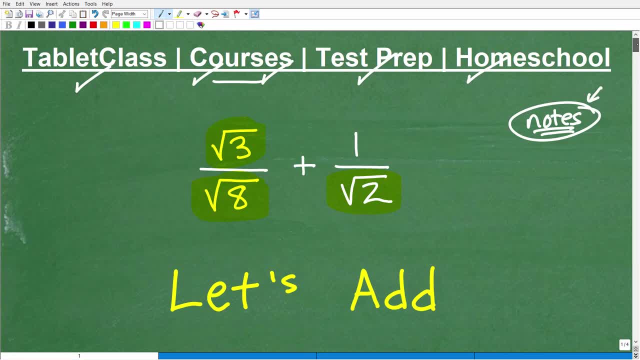 you're going to be. So you know, the more math you know, the better off you're going to be. Okay, There's not. you know, generally speaking, in math there's not just one way to do a problem. All right, So hopefully this was a good little review. Again, if you're still having